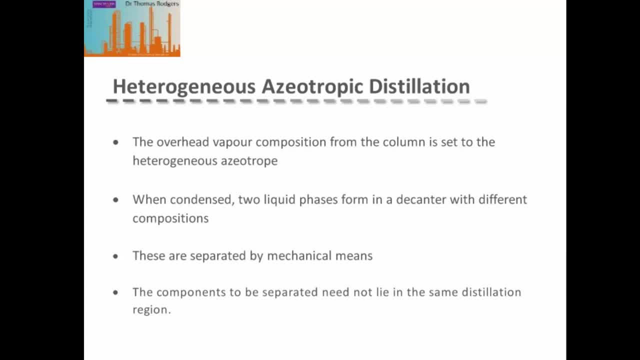 lie in different distillation regions of the residue curve map, then the restriction on heterogeneous azeotropic distillation is generally overcome. And in fact, with heterogeneous azeotropic distillation, because of the compositions of these two liquid phases, the components that we're actually separating do not need. 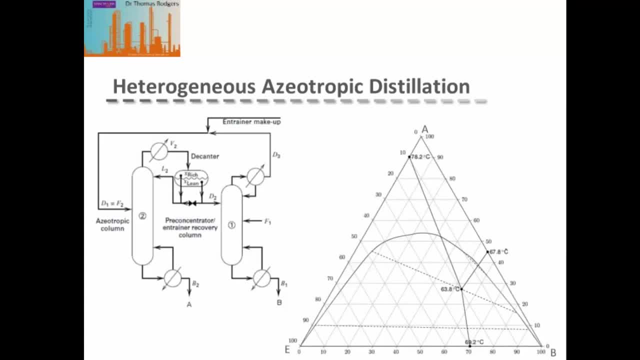 to actually lie in the same distillation region. So on the right hand side we have our ternary diagram that shows both our distillation regions and our liquid-liquid two phase region. The distillation regions are given by the straight black lines. 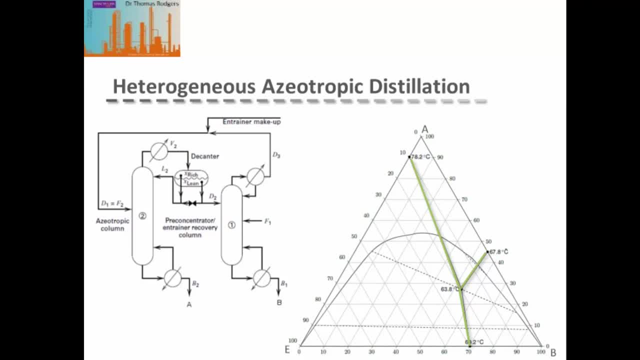 Joined by the points with temperatures, And these points are the azeotropes and the temperatures are the temperature of the azeotrope. Our two phase region is given by our curve, with the liquid-liquid equilibria given by the dotted tie lines between them, And we also 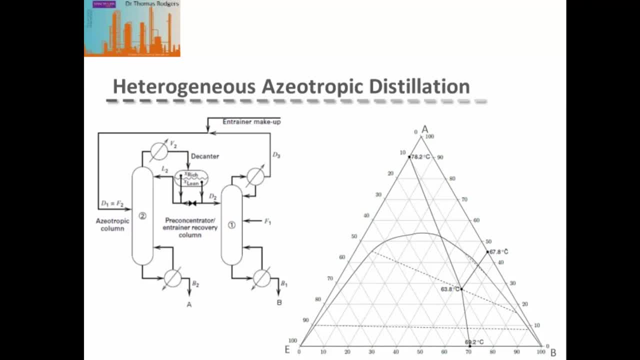 have one tie line that passes through our ternary azeotrope. that actually gives us the liquid-liquid equilibria for a liquid composition. at our ternary azeotrope, On the left hand side, we have a common two column system set up for heterogeneous azeotropic distillation. 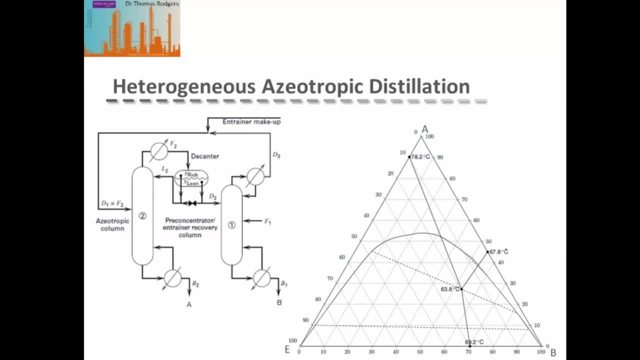 And you can see in this case that both of the columns have multiple feeds. But as it's difficult to draw columns with multiple feeds on the ternary diagrams, we can actually split this up into mixing points before the column and then columns with a single feed. This 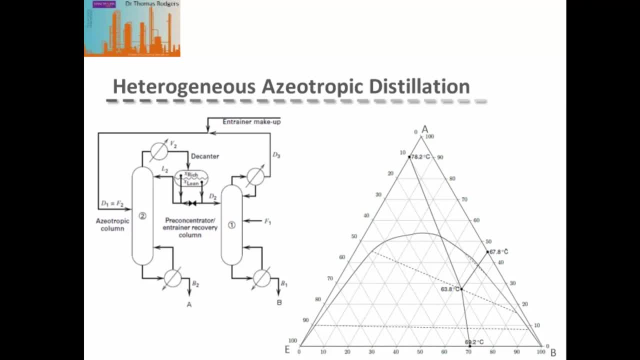 doesn't affect in any way the separation. It just affects the ternary diagram, The final design of the system. So what we can do is we can separate our two multiple feed points into our new system. On the left hand side we now have that redrawn system. 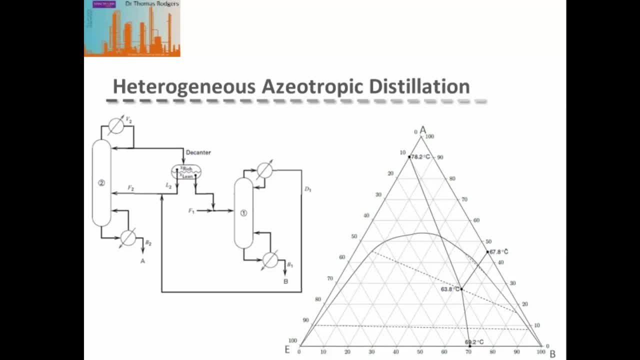 with our mixing points and our single feeds to the columns, But it is identical in terms of separation feed points to our previous system And after we've actually calculated that, you can actually transform that back into the previous system to allow you to fully design the actual, better designed industrial system for heterogeneous separation. 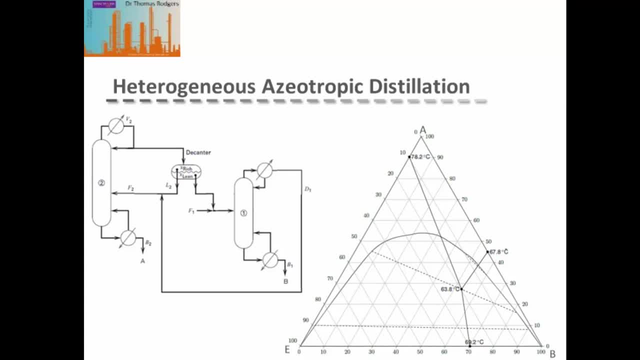 If we're trying to draw this system on our ternary diagram, we need to start with information that we know about our system. So we know that for heterogeneous azeotropic distillation, what we try and do is get the top product of one of our distillation columns to be approximately 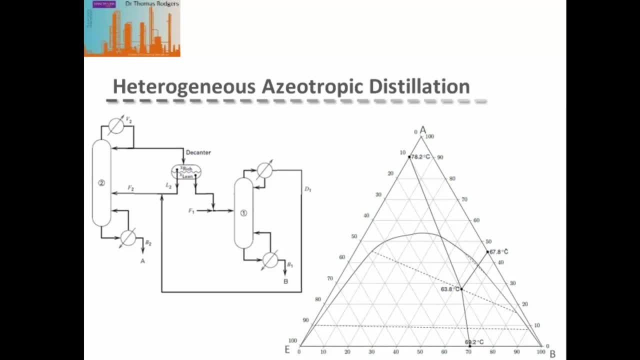 equal to the heterogeneous ternary azeotrope. So we can define the separation in our decanter by the tie line that passes through this ternary azeotropic point. So we can show this by the red line. We also know the feed composition of our system, So in this case we can just 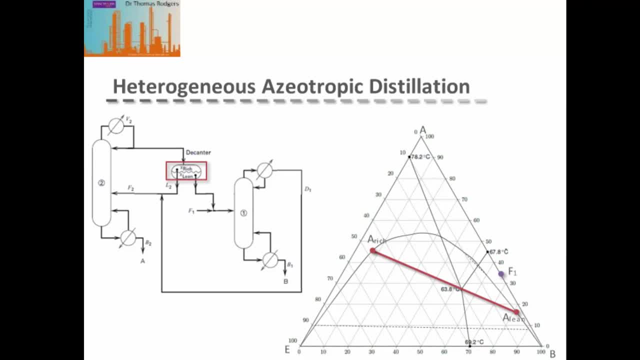 represent that as a point F1.. We know that we then have mixed feed points. This is our lean liquid phase with our feed point, And we know this is represented by a straight line, So we can draw this on as a green line between these two points. 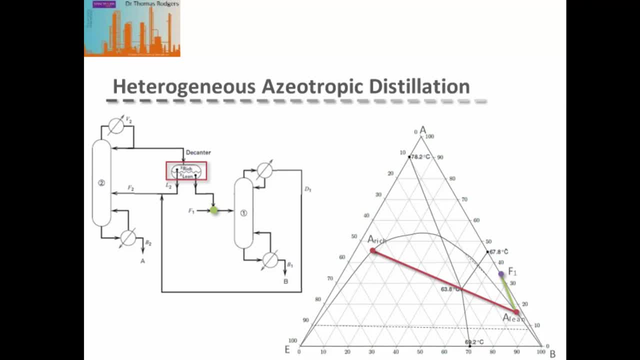 In our second distillation column we want to achieve a separation that gives us some of our B as a pure component. Now we know we have to do this in this column because our feed is in the distillation region that allows us to get pure component B. 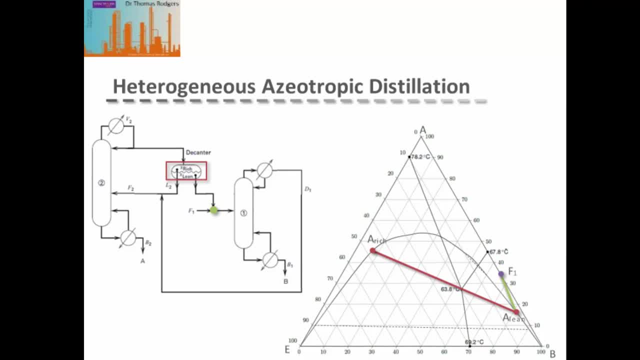 We can draw a straight line from our pure component B that passes somewhere through our green mass balance line for the mixing point up to a distillate product. Now, if this diagram had residue curves on it, which it can do, we would know where we. 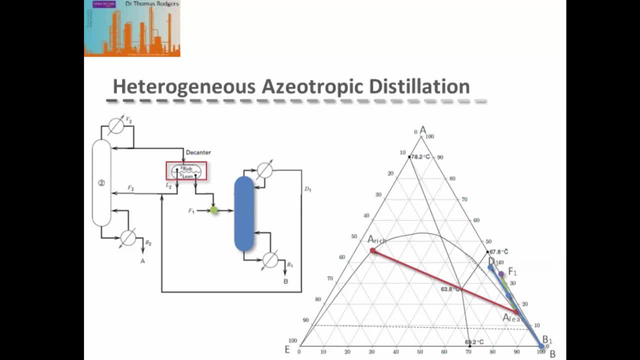 can put our distillate composition. However, if I did have residue curves on this diagram, it would be even more difficult to see what was going on, So I've left them off And therefore I've just gone up to an approximate point D1, representing about where it would. 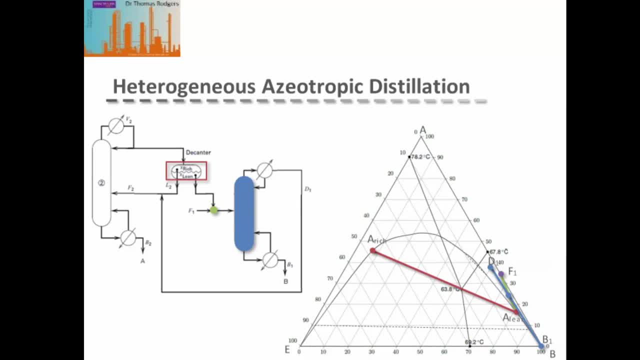 be with our residue curves. We now know from our system that what we want to do is we take this D1 composition and we mix it with our rich phase from our decanter. We can again represent this as a green line between our point A- rich.